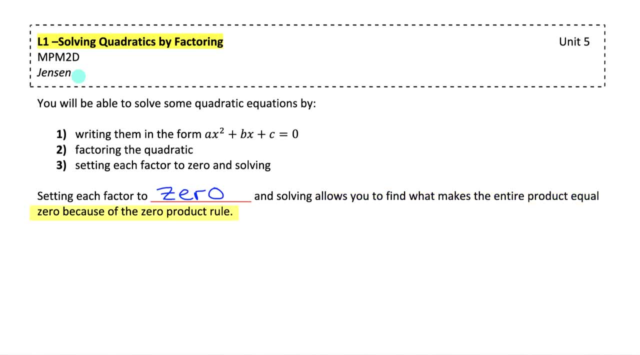 allows you to find what makes the entire product equal to zero because of the zero product rule. And why do we care? what makes the product of the factors be zero? Well, as long as we followed step one, we know that what we're trying to find the quadratic is equal to is zero. So if we get it, 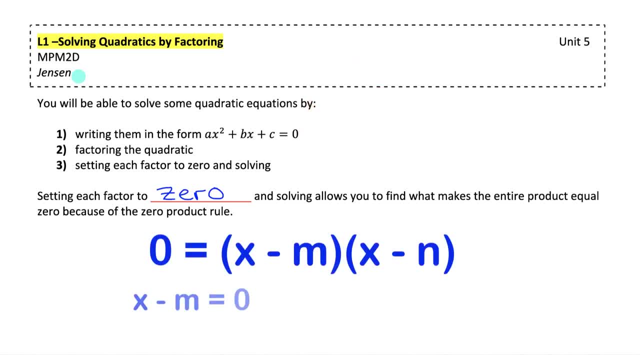 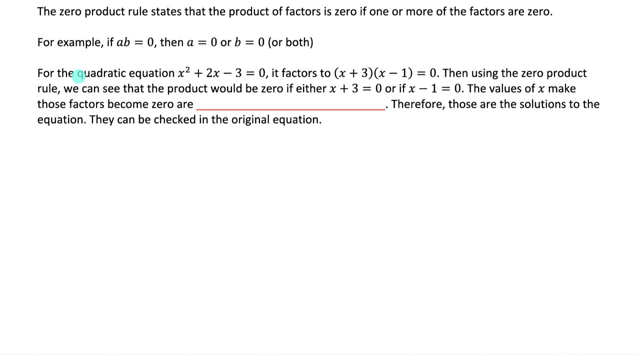 written as a product of factors and then determine what values of the variable make either of the factors be zero. we've essentially solved the equation because we're interested in what makes the equation be zero. Now I mentioned something called the zero product rule. What is the zero? 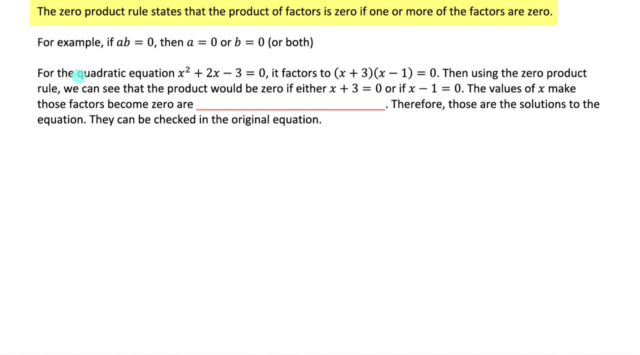 product rule. The zero product rule states that the product of factors is zero if one or more of the factors in the product are zero. For example, if a times b equals zero, then I know that either a is zero or b is zero, or both. 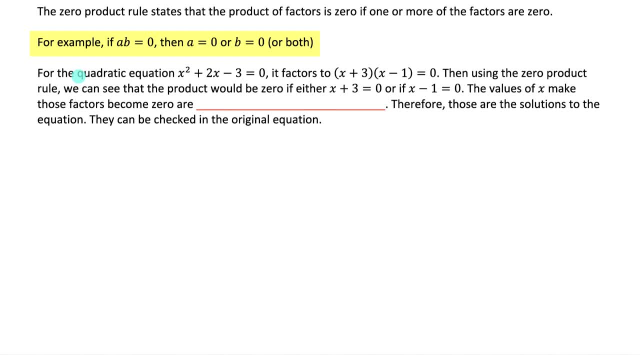 That's the only way that this product could be equal to zero is if one or both of the factors are equal to zero. How does that apply to quadratic equations? Well, for the quadratic equation, x squared plus 2x minus 3 equals zero. I know that that would factor to x plus 3 times x minus 1. 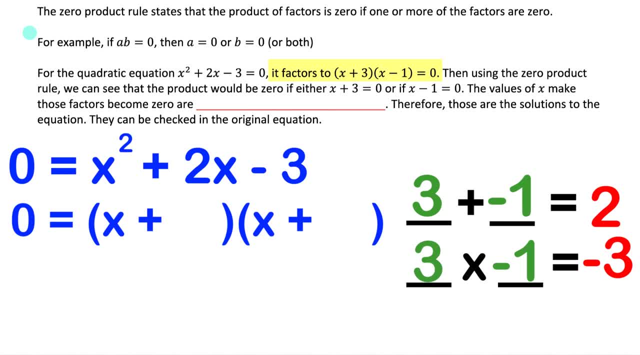 equals zero because 3 and negative 1 are the numbers that multiply to negative 3 and add to 2. They satisfy the product and sum we would need to find to factor The quadratic on the left side of the equation Once we have a product of things equal to zero. 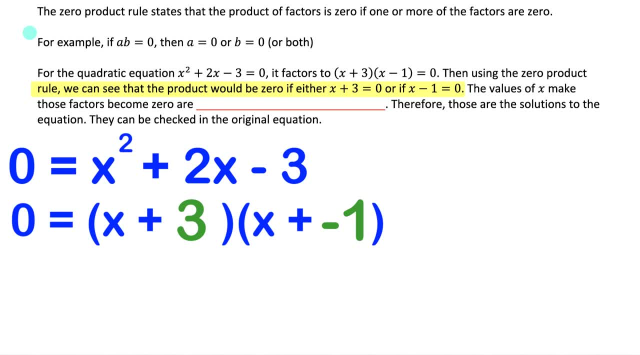 the zero product rule says the product of those factors would be zero. if either of the factors- the x plus 3 or the x minus 1, were equal to zero, The values of x that would make those factors become zero are: well, what would make x plus 3 equal to zero? An x value of negative 3. 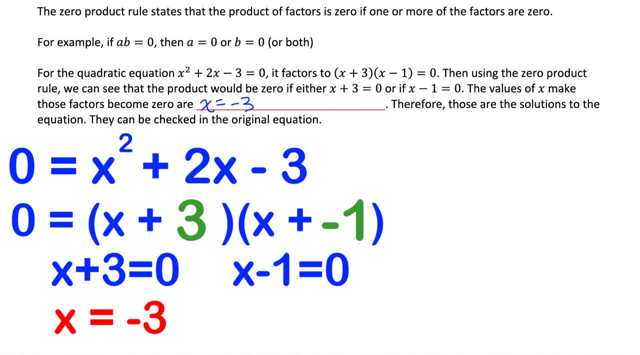 would make x plus 3 be zero. It would make x minus 1 be negative 4, or to plug in negative 3 for both the x's. in my factored form equation I would have zero times negative 4, which is zero. So that is an answer to the equation And you can also check it in the 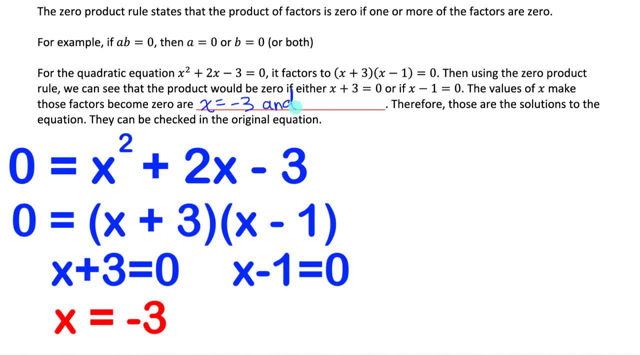 standard form equation as well to verify. But don't forget, the zero product rule says that the product would be zero if either of the factors are zero. Well, I know negative 3 would make the first factor be zero, but what would make the second factor be zero? Well, x minus 1 would be. 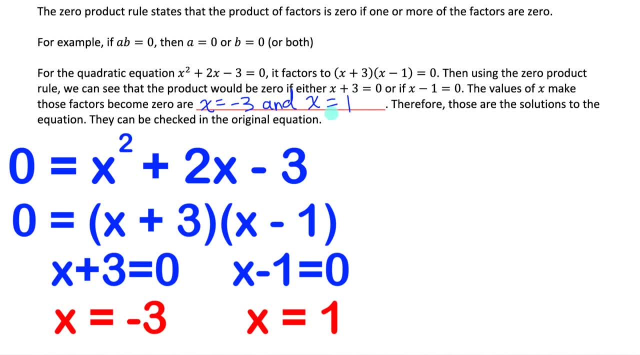 zero if x was 1.. So that would be 0. And then I would have x minus 1,, which would make x minus 1, equal to 1.. If x was 1,, if we subbed that into the factored form equation, I would have 4 times zero. 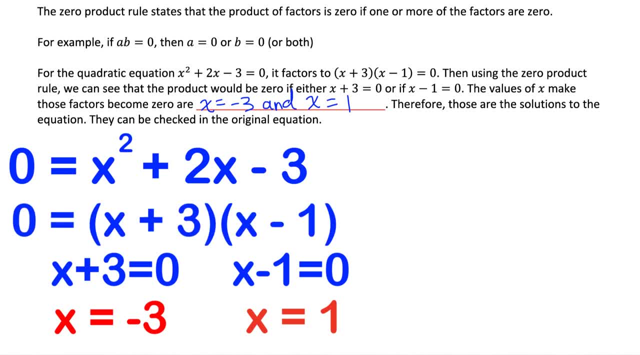 which of course equals zero. So x equals 1 is also a solution to the equation And, like I said, you could sub that into the standard form equation as well, to verify that it satisfies that equation. Keep in mind: anytime we're solving an equation, all we're trying to do is figure out what value. 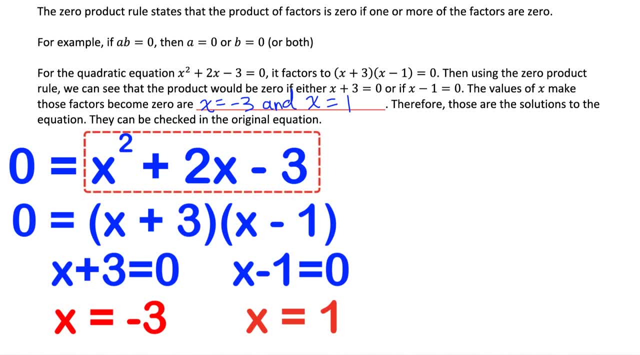 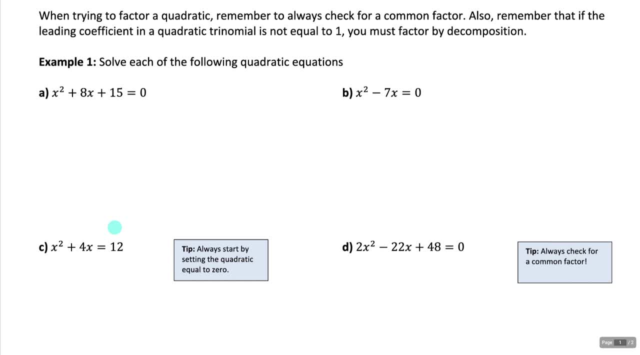 the variable makes the left side of the equation equal to the right side of the equation. And before we get started with an example, I just made a note here of a couple tips you should remember. When trying to factor a quadratic, remember to first always check for a common 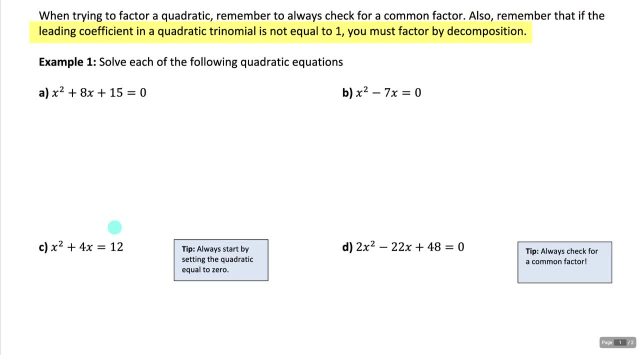 factor. Also, remember that if the leading coefficient in a quadratic trinomial is not equal to 1, so if the a value is not 1, we have to factor by the method of decomposition And that'll come up, as we do examples here. so I'll have a chance to remind you of what that. 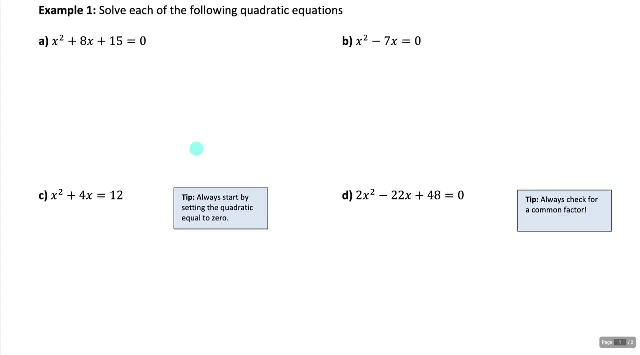 looks like All right. finally, let's get started. So let's start with the first factor. So let's get to an example. Let's look at example one. It says to solve each of the following quadratic equations: The highest degree term in all of these equations is degree 2.. That's what makes 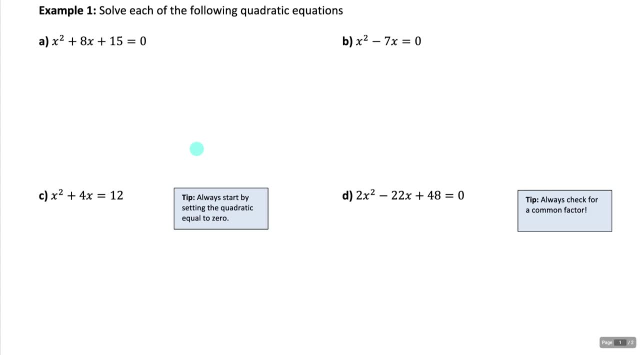 them quadratic And we want to figure out what value of the variable. in this case the variables are all x's, so what values of x make the left side of each of these equations equal to the right side? Step number one, if we look at a, is going to be making sure that we have one side of 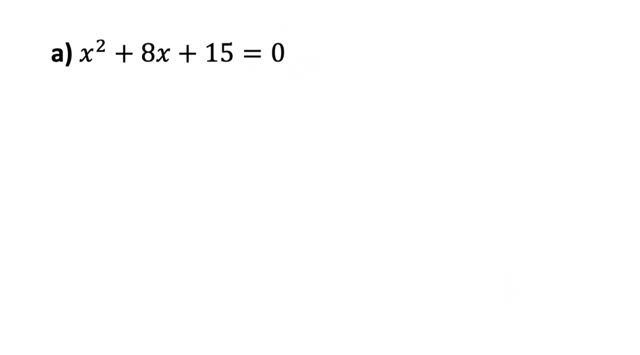 the equation equal to zero. So make sure all of the terms are moved to one side. All of the terms are already moved to the left and the right side is equal to zero. so step one is done. Step two says to factor the quadratic, Because we have a three-term quadratic where 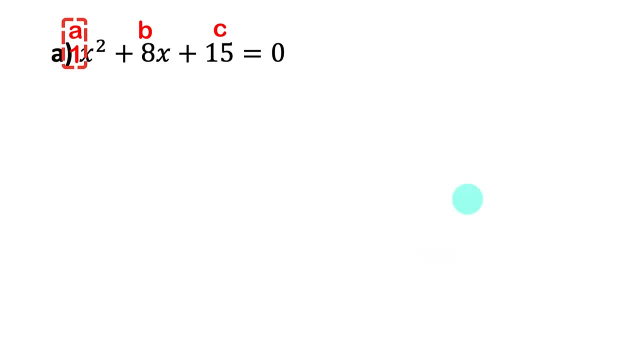 the leading coefficient. the a value is 1,. I can factor it by finding the numbers that multiply to the c value. so in this case, multiply to 15, and add to the b value, in this case 8.. The numbers: 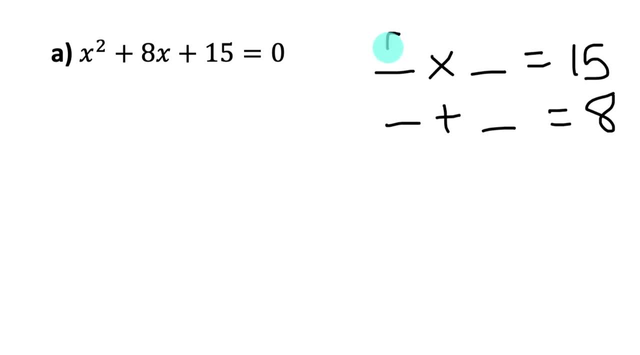 that multiply to 15 and add to 8 are 4.. So we have a 3-term quadratic where the leading coefficient is 5 and 3.. 5 times 3 is 15, and 5 plus 3 is 8.. This will allow me to rewrite the left side of the. 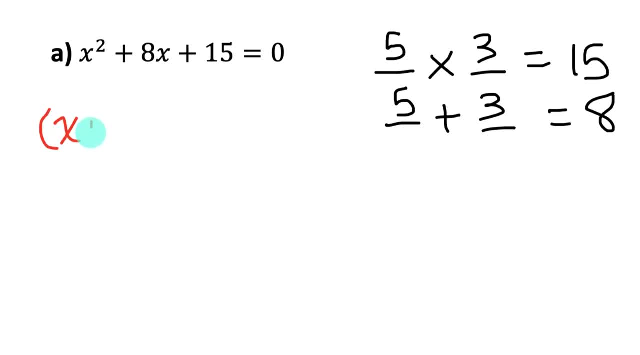 equation in factored form. The factored form would be x plus 5 times x plus 3 equals 0. Now that I have it in factored form, now that I have a product of two things equal to zero, I know that product. 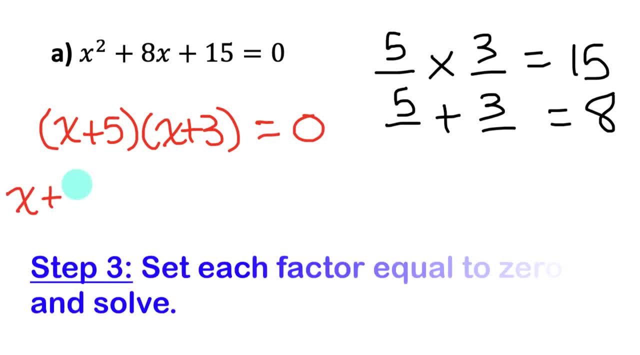 would be zero if either the first factor was zero, so I'll write x plus 5 equal to zero, or if the second factor was equal to zero, so I'll write x plus 3 equals zero. and then I'll solve each of those equations I've made to figure out what value of x would make each of those factors. 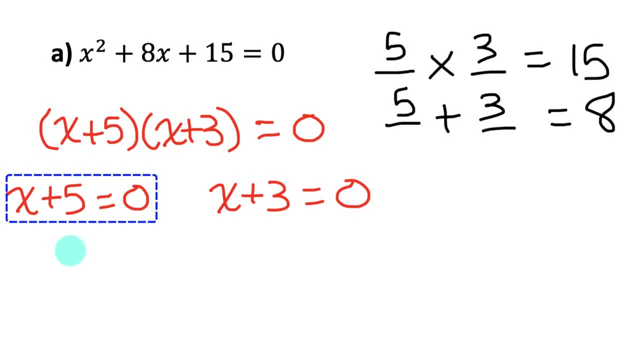 be zero. If I solve the first equation by moving the plus 5 to the other side, I would have x equals negative 5,. and if I solve the second equation, take the plus 3 and move it to the other side, I would have x equals negative 3.. So my answers are x equals negative 5,. 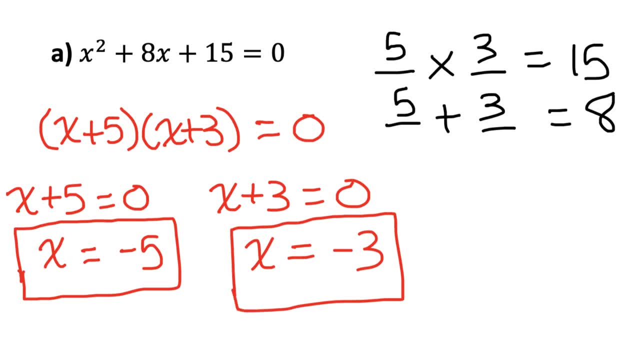 and x equals negative 3.. When you have multiple answers for your variable, sometimes you'll see a subscript number beside the variable indicating which numbered solution it is. My first solution was negative 5,, so I'll say x1 equals negative 5, and my second solution was negative 3, so I'll 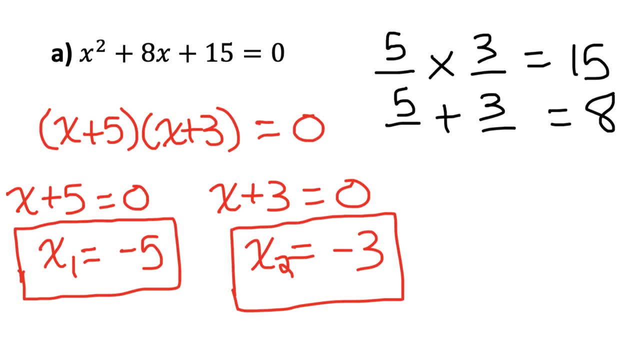 say x2 equals negative 3. Make sure you remember that you can actually check these answers in the original equation to make sure it makes the left side equal to the right side. In fact you should always do a left side, right side check just to make sure that you have the right side, right side. 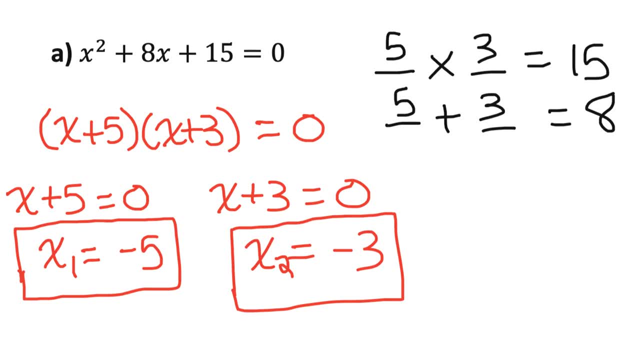 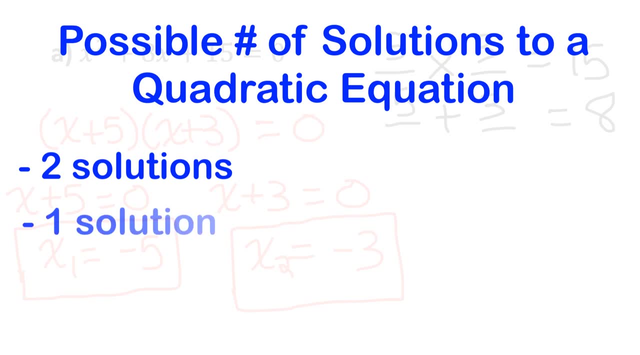 to satisfy the original equation. And I should note that when solving quadratics you're not always going to get two answers. Sometimes you'll get one, sometimes you'll get zero. and we'll talk more about those possibilities as we go through the unit. Let me actually just quickly show you. 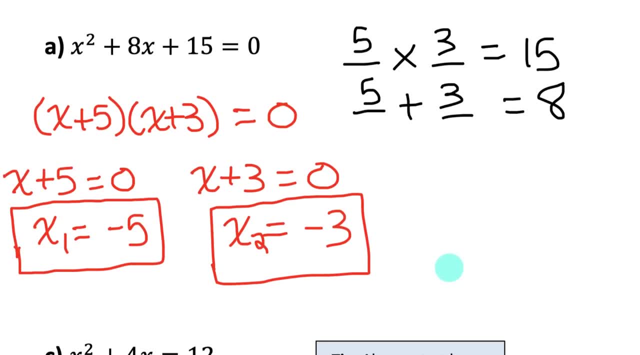 a left side, right side check to verify the answers for a. We won't do that for all the questions, but I just want to make sure you understand how we would do that. Notice, if I sub negative 5 in for the x's in the original equation I'm going to have x equals negative 5, and I'm going to. 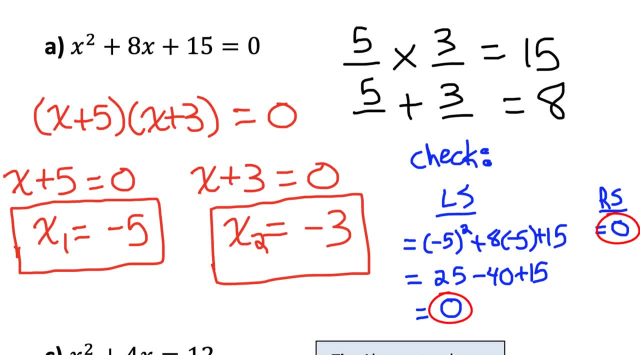 make sure that the left side of the equation is equal to zero, just like the right side of the equation. so negative 5 is the correct answer. And if I sub negative 3 in for the x's in the original equation, it makes the left side equal to zero, just like the right side. so that's the 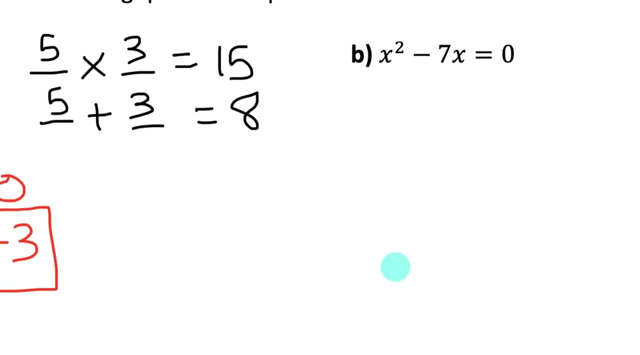 correct solution as well. Let's move on to part b. Notice for part b. once again, all the terms are already to the left side of the equation. The right side of the equation is equal to zero, so step one is done. 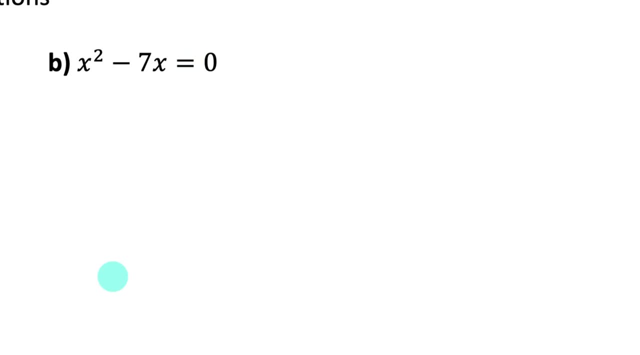 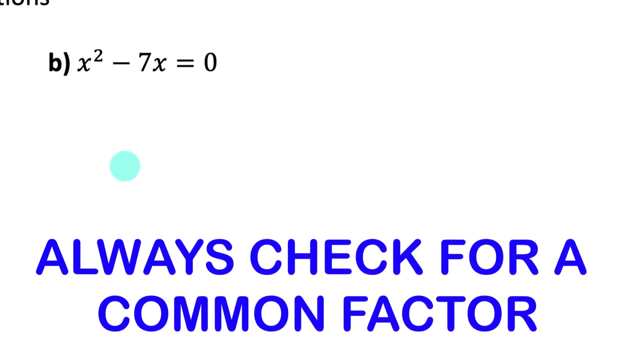 But this quadratic is only two terms so I'm not going to need to do any product and sum factoring. In fact, because there's no constant term, I notice that both terms have an x. So what I should do to get this into factored form is just: common factor, out an x from both terms. on the left side. 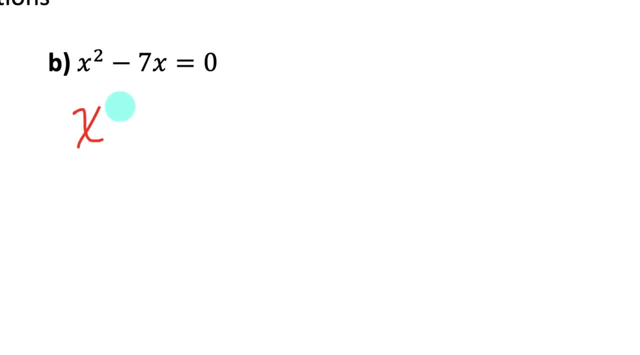 of the equation. So I'll take out a common factor of x and then, in brackets, divide both of the terms by the x. I'm common. factoring out: x is x minus 7x divided by x is 7.. So the factored form is x multiplied by x minus 7.. The product of 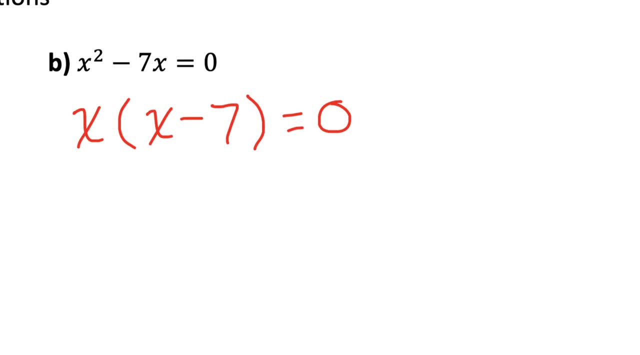 those two factors would equal zero if either of the factors were zero. So I'll set each of the factors to zero and solve. My first factor is just an x, so if I set that to zero, that equation's already done. What would make x be zero is: if x was zero. 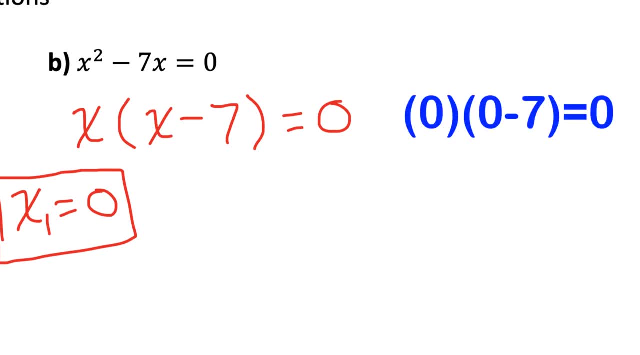 My second answer is zero. If we think about plugging in zero into my factored form, I'd have zero times negative seven. That's zero. What if my second factor was zero? x minus seven would be zero if x was seven. If I plug seven into my factored form, I'd have seven times zero which. 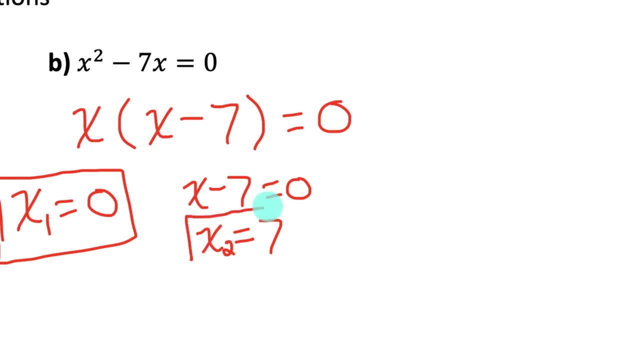 is also zero. So my second answer is seven. Now we should also check those answers into the original answer. So if I plug seven into my factored form, I'd have seven times zero, which is also zero. So I'll use the original equation to make sure it works to satisfy the original. 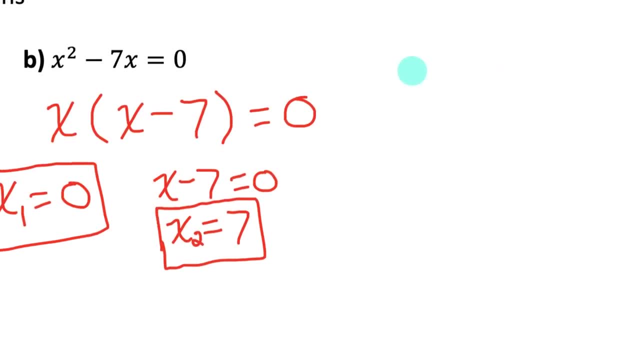 equation. If I check my first answer of zero, this is what it would look like. Notice that zero satisfies the original equation. It makes left side and right side both be zero. Now let me check seven. Seven also makes both sides of the equation equal to zero, so seven is also a correct answer. 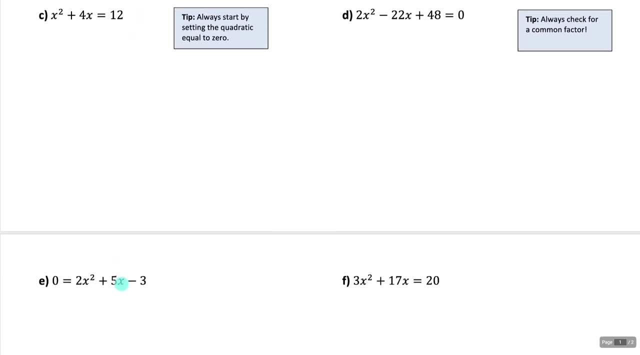 to the original equation. Let's move on to part c. Notice in part c: this is the first time where we've had a quadratic equation Where it's not set equal to zero. So the first thing we're going to have to do is rearrange this. 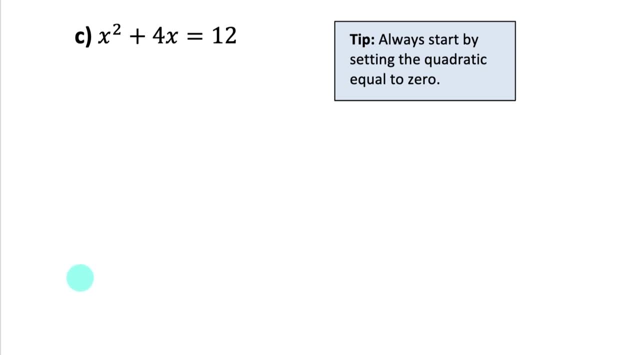 quadratic by moving all terms to one side so that it is equal to zero. What I'm going to do is I'm going to take that constant of 12 that's on the right and subtract it over to the left side of the equation. That would give me x squared plus 4x minus 12 is equal to zero. And now that the 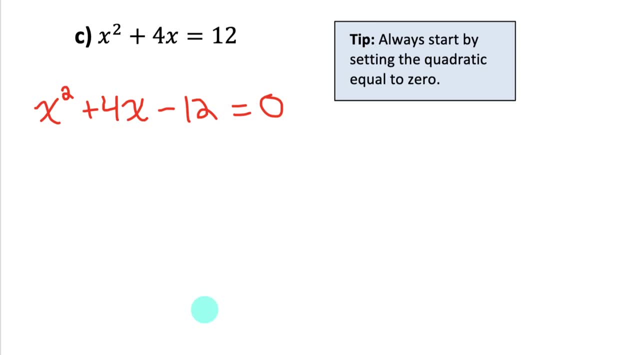 quadratic is equal to zero. we'll try and factor it, Because the quadratic has three terms and the leading coefficient, the a value, is one. I'll need to find two numbers that have a product of the c value negative 12, and a sum of the b value four, The numbers that satisfy that product. 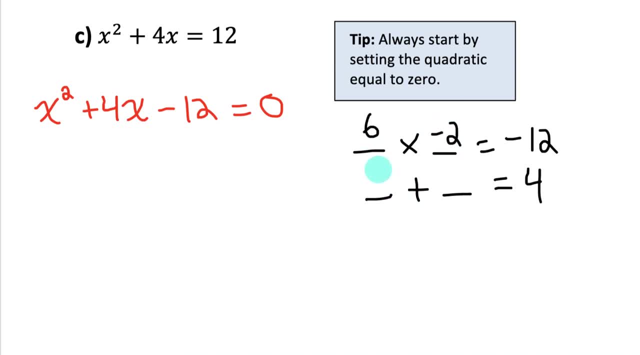 and sum are six and negative two. Six times negative two is negative 12.. Six plus negative two is four, The factored form version of the quadratic x plus six times x minus two, And that factored form quadratic is equal to zero. We want it equal to zero because it's very easy to determine when a 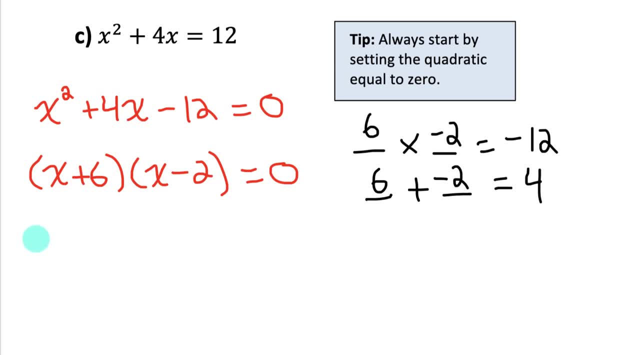 product is equal to zero. A product of two factors is zero if either of the factors is equal to zero. So we set each of the factors to zero and then solve within each of those two equations what values of x satisfy those two equations. 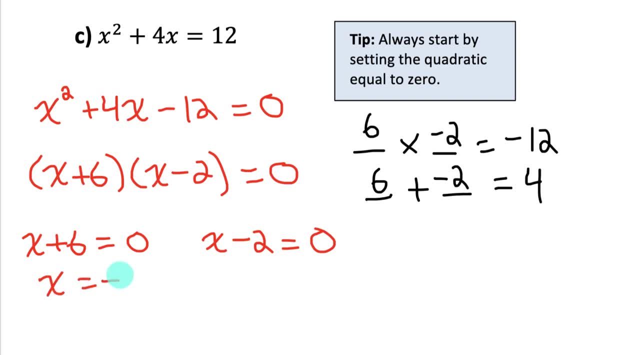 x plus six would equal zero if x was negative six. So that is my first answer to this equation. And my second answer would be: what makes x minus two equal to zero? would be if x was equal to two? So my second answer is: x equals two. Make sure you remember that you could check both of those answers into the original equation. 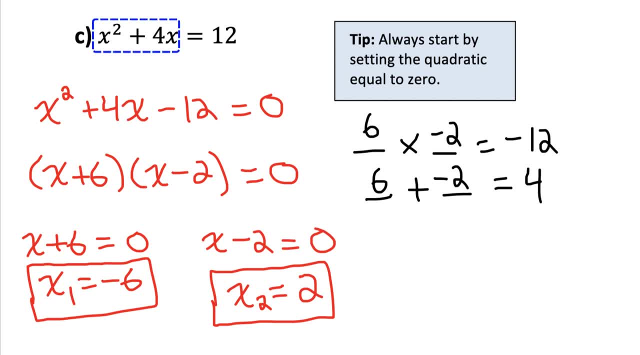 Both of those answers should make the left side of the equation equal to 12, so that it matches the right side of the equation. And I hope at this point you're also fully grasping the zero product rule, Understanding why negative six and two are both solutions. 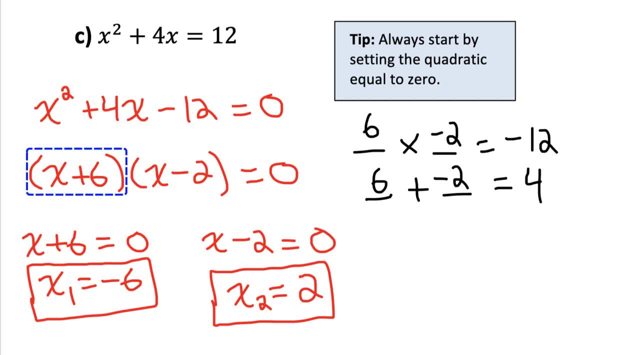 Because those values are what would make either of the factors in the factored form equal to zero. Right, I know, the value of two would not make the first factor be equal to zero, it would make it be equal to eight, But it would make the second factor be zero. So we would have eight times zero, which is zero. 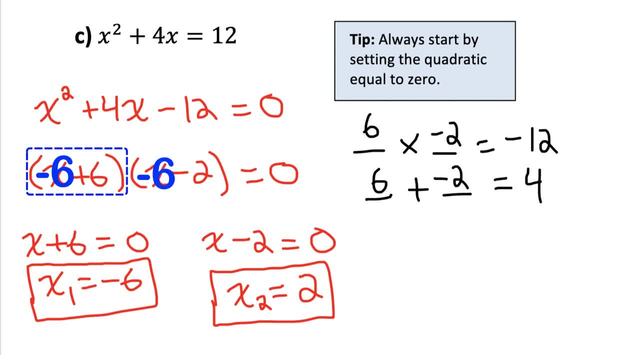 And negative six would make the first factor be zero, but not zero, Not the second. It would make the second factor be negative eight. but zero times negative eight is zero. So as long as we can find a value of x that makes any of the factors be zero, that is an answer to the equation. 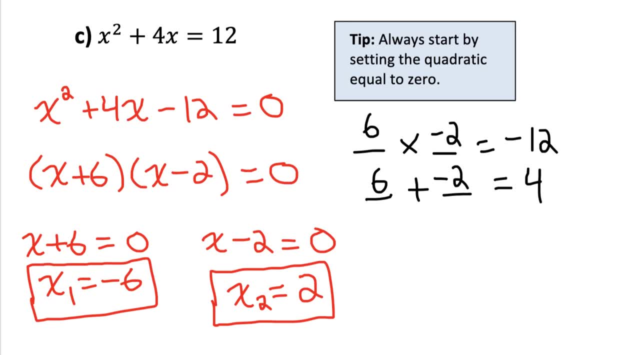 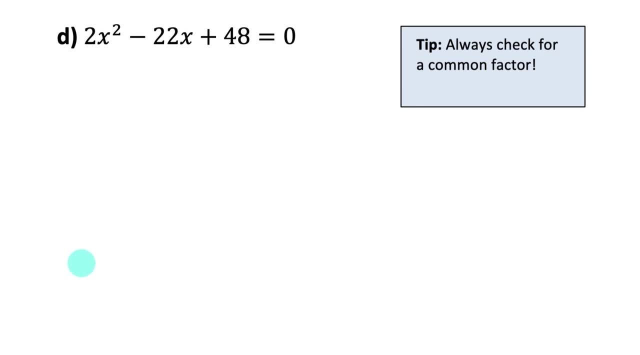 As long as your factored form is set equal to zero, which is what we take care of at the beginning of the question. Let's now move on to part d, Part d- Notice I put a tip off to the right there: Always check for a common factor. It'll make the question a lot easier if we're able to common factor out. 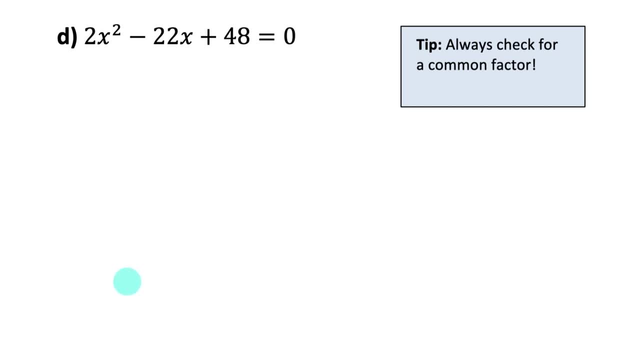 The leading coefficient of the quadratic. I should also mention that what we have here is a quadratic set to zero, so all the terms are already moved to one side. Check for a common factor. I can common factor out a two from all of the terms. 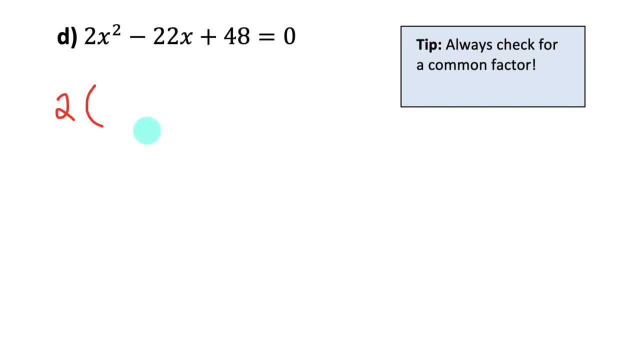 So I'll take out two as the first factor and then divide each of the terms by two to get my second factor. That would give me x squared minus 11x plus 24.. And now, if I focus inside the brackets, I notice it's a quadratic with three terms. 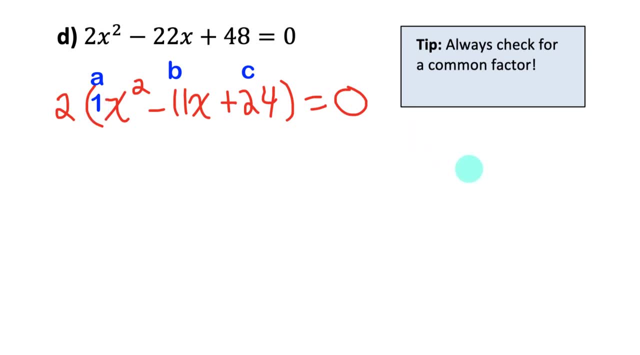 The leading coefficient, the a value, is one. So once again I need to find numbers who have a product of the c value, So a product of 24. And a sum of the b value, So a sum of negative 11.. 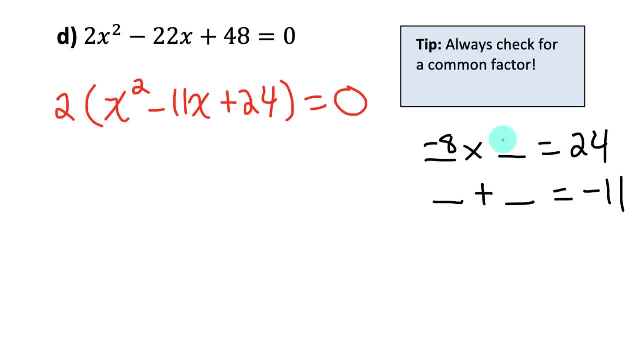 The numbers that satisfy that product and sum would be negative 8 and negative 3.. Negative 8 times negative 3 is 24.. Negative 8 plus negative 3 is negative 11.. That would allow me to factor the quadratic. If it's in brackets, I could factor it to x minus 8 times x minus 3.. 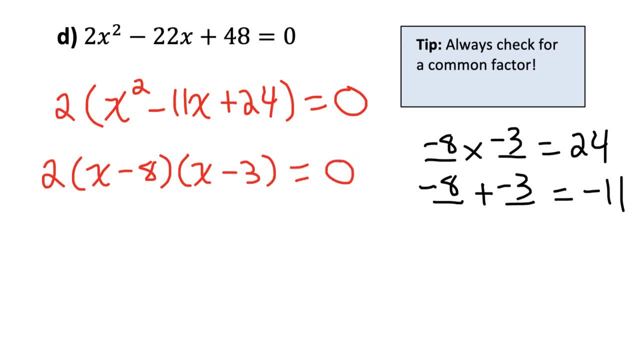 Notice that factor of two is just staying out front. If we wanted to, I suppose we could divide it to the other side to eliminate it, but it's not going to hurt anything staying there. So now I have a product of three factors equaling zero. 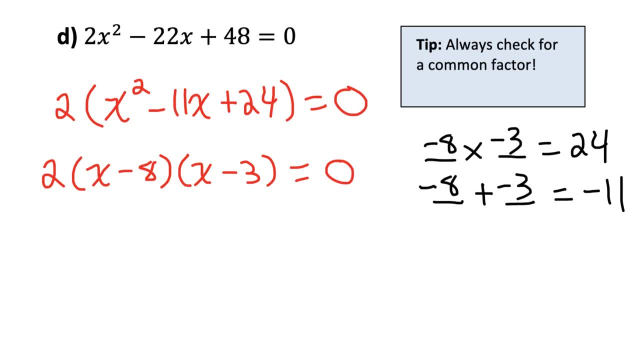 Well, the product of those three factors would be zero if any of those three factors were zero. So let's look at. how could any of those factors be zero? Well, my first factor is two. Can two be zero? No, two is a constant. 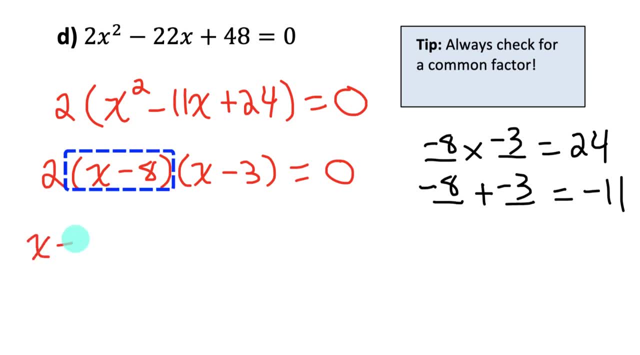 It's always two. But could x minus eight be equal to zero? Yes, that would be equal to zero if x was equal to eight. So my first answer is eight. It would make my factored form say two times zero times five, which is zero. 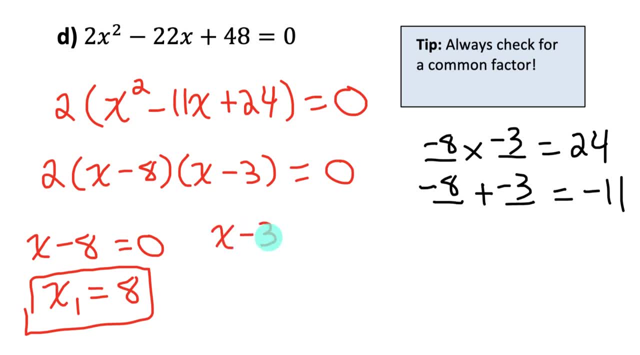 And if we look at the last factor, x minus three, that would be equal to zero if x was equal to three. So my second answer is three. It would make the factored form say two times negative, five times zero, And that's zero. 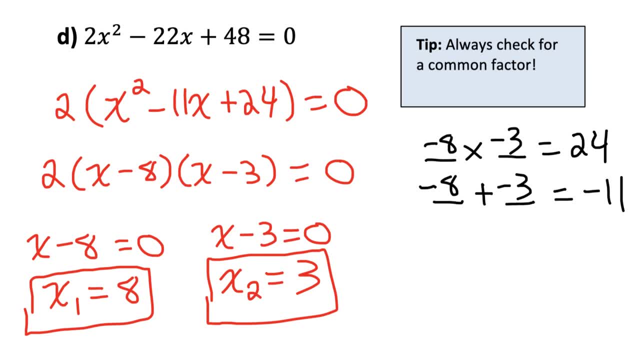 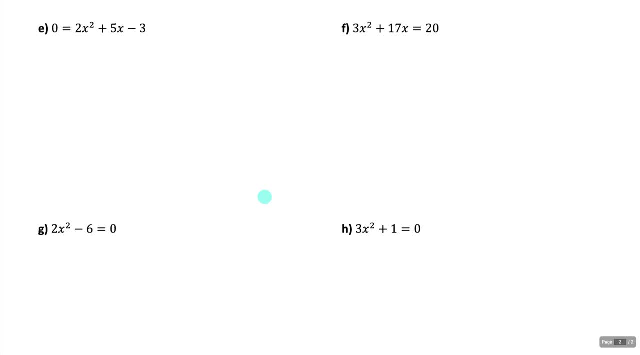 So that's an answer to the equation And once again you should take the time to check those in the original equation to make sure it makes left side equal to right side. Okay, we have four more quadratics to solve Part e. all the terms are already on one side and the other side is equal to zero. 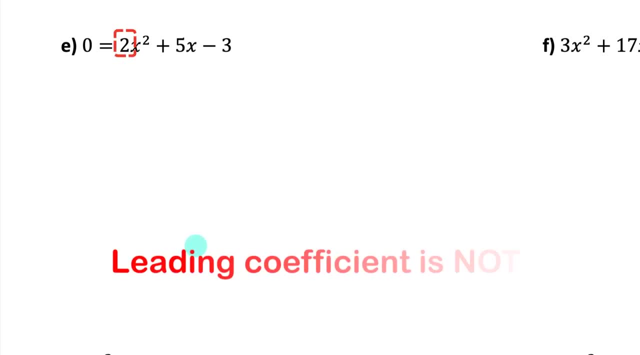 It's a three-term quadratic where the leading coefficient is not one, it's a two. but this time I can't common factor it out because two doesn't go into five and three. So to factor this quadratic we're going to have to do it using the method of decomposition. 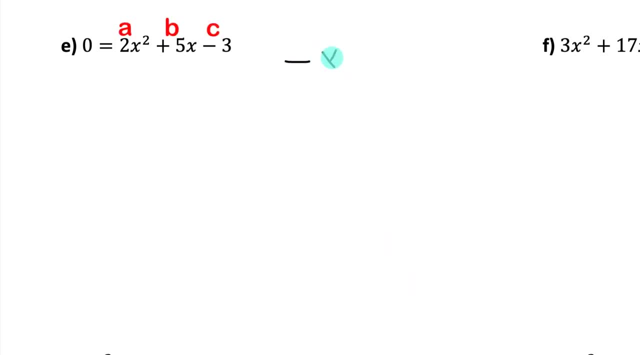 While using that method, we find numbers that have a product of not just the c value but of a times c. So two times negative three is negative six And a sum of the b value which is five. The numbers that multiply to negative six and add to five would be: 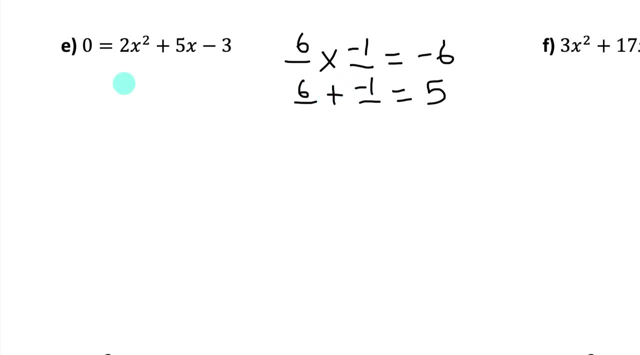 six and negative one. And because the leading coefficient of a value is not one, what we have to do is split the middle term, that five x. we have to split it into six x minus one x. We split it into those two values: six x and negative one x. 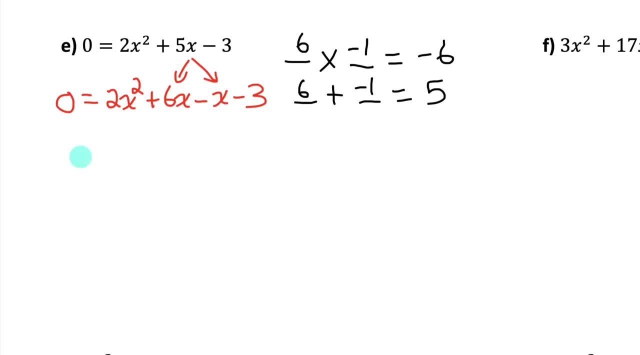 because those are the numbers that satisfy the product sum. And now what we do is we look at the first two terms and take out a common factor Between the first two terms. I could common factor out a two x. When I divide the first two terms by two x, I get x plus three. 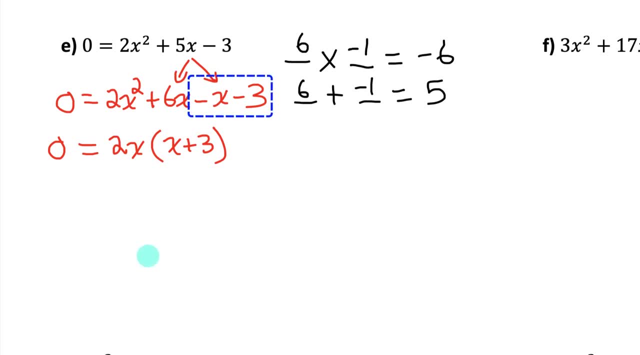 I then look at the last two terms, my negative one, x, and my negative three, And what I could common factor out from those two terms. well, when the first term in a group has a negative, we definitely have to factor out at least a negative one. 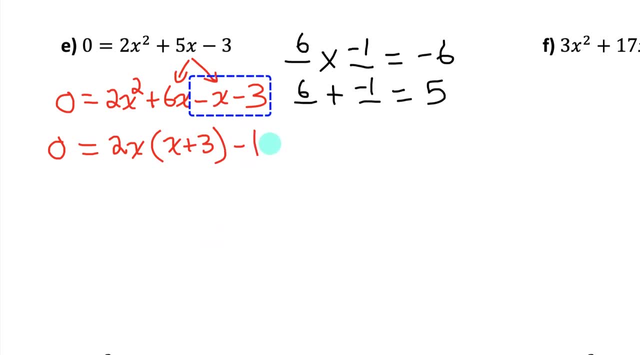 And in this case that would be the greatest common factor between those two terms. When I divide the negative x and the negative three by negative one, that gives me x plus three. Notice I have a common binomial: Both terms have an x plus three. 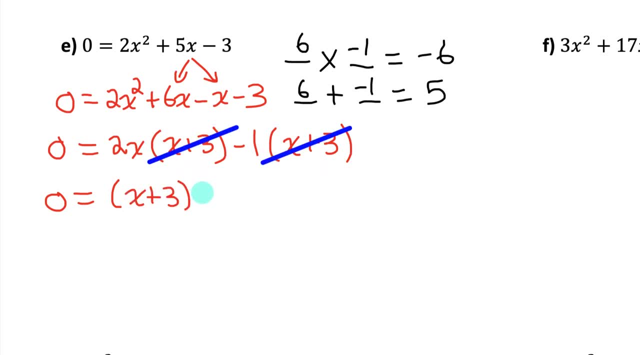 So I factor out an x plus three from both terms, And what I'm left with when I divide both terms by x plus three is two x minus one. It's now into factored form. So I know the product of those factors is zero. 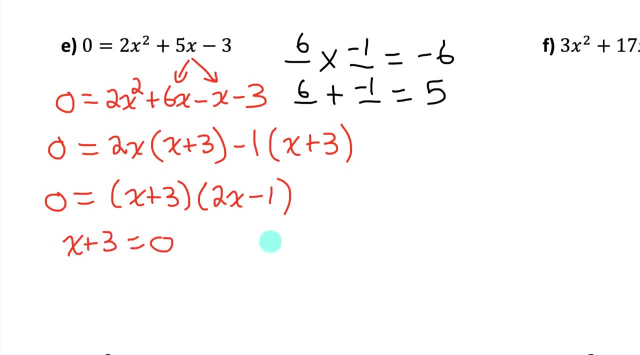 if either of the factors is zero. So I'll set each of the factors to zero And solve each of the equations. The first equation is easier to solve: Just move the plus three over. We get x equals negative three. That's my first solution. 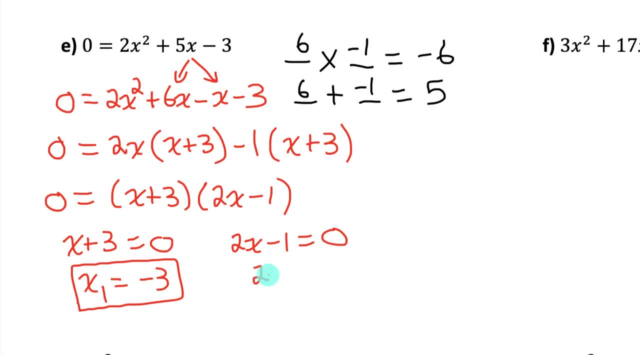 When solving for when the second factor is zero, it'll be two steps: Add the one to the other side And then divide the two. So I would get my second answer is: x equals a half. Part f is going to be just like part e. 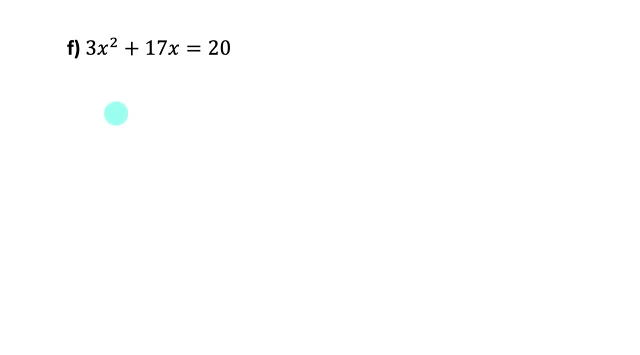 But notice it's not set equal to zero to start. So our first step is going to be moving to the other side of the equation. Notice it's a three term quadratic. The leading coefficient, the a value, is not one, It's a three. 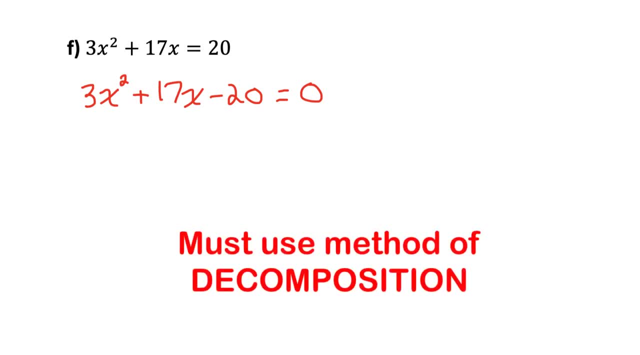 And we can't common factor out the three. So once again we're going to have to do this the long way by decomposition. We'll need to find numbers that have a product of a times c, So a product of three times negative twenty. 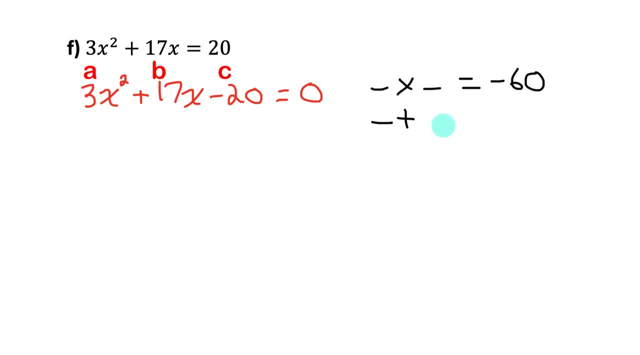 Which is negative sixty, And a sum of the b value seventeen. The numbers that satisfy that product and sum are twenty and negative three. So, once again, because the leading coefficient was not one, we have to factor this by the method of decomposition, where we split. 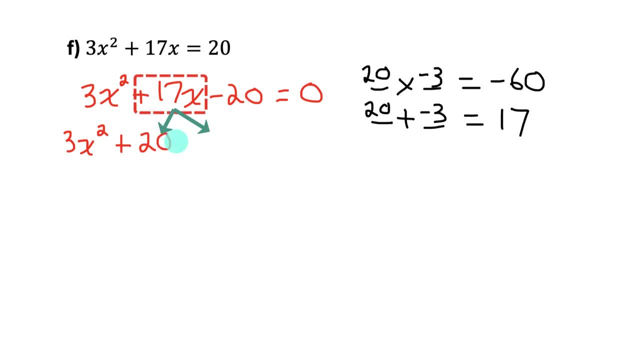 the middle term. we split that seventeen x into twenty x minus three x, And then we look at the first two terms and take out a common factor. All I could take out is an x from the first two terms and that would leave me with three x plus twenty. 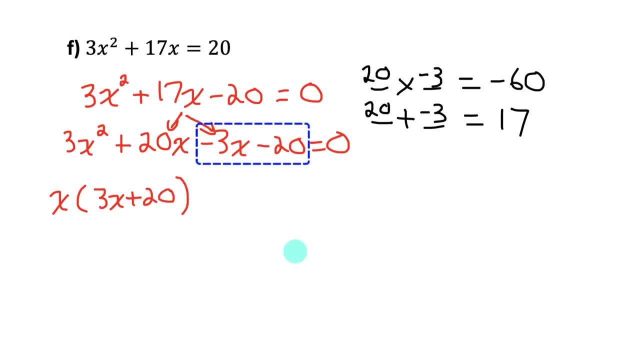 And then the last two terms, the negative: three x minus twenty. all I could take out is a negative one, And when I divide the last two terms by negative one, I get three x plus twenty. Notice I have a common binomial. 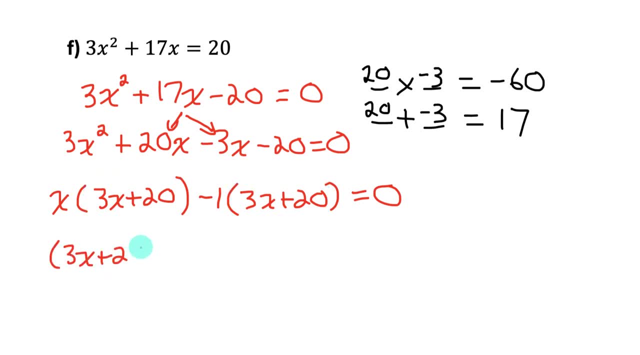 Both terms have a three x plus twenty. So I'll common factor out that three x plus twenty, And when I divide both the terms by that binomial I'm left with x minus one. Now I have a factored form quadratic equal to zero. 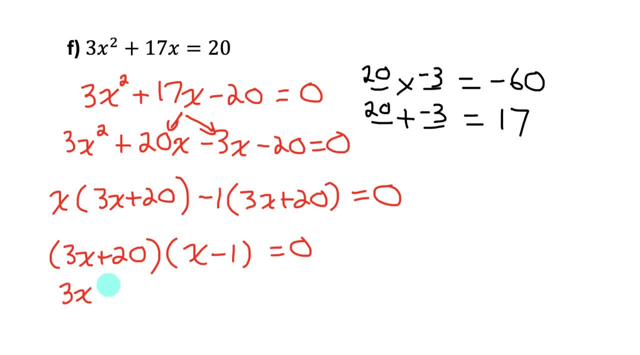 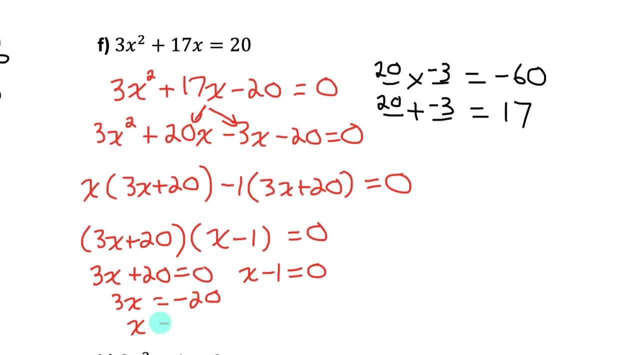 That product would be zero if either of the factors were zero. So set three x plus twenty, equal to zero, and set x minus one, equal to zero, and we'll solve both of those equations. The first one will be two steps: Subtract the twenty over and then divide the three. 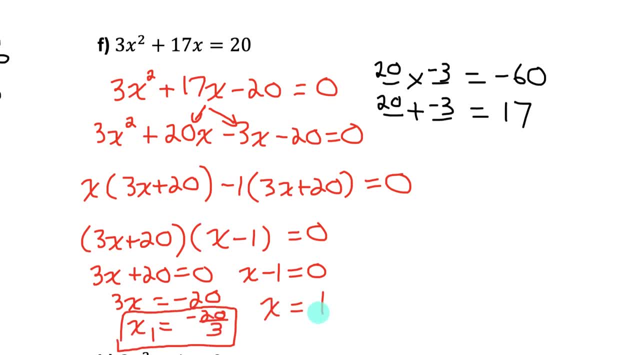 The second one. just add the one over and we get my second answer is x equals one. So my answers are negative: twenty over three and one. And once again, don't forget, you can check those answers in the original equation to make sure they're correct. 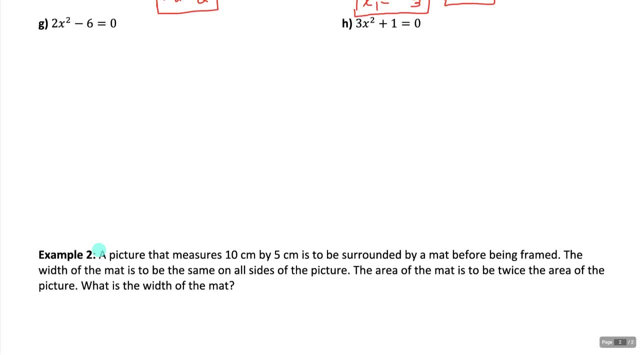 We have two more quadratics to solve before we do a short application question. These ones are a bit different because- notice- they're only two terms. They have the degree two term and the constant. When we have an equation like this, we're actually not going to solve it by factoring. 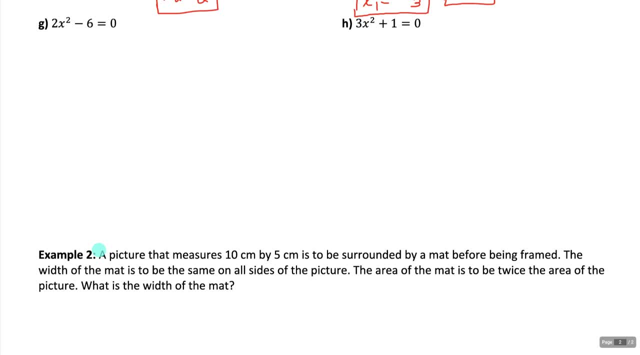 It'll be easier for these ones if we actually just try and isolate the x using normal algebra. There's only one term that has an x, So let's just use algebra to try and isolate that x In part. I would just start by 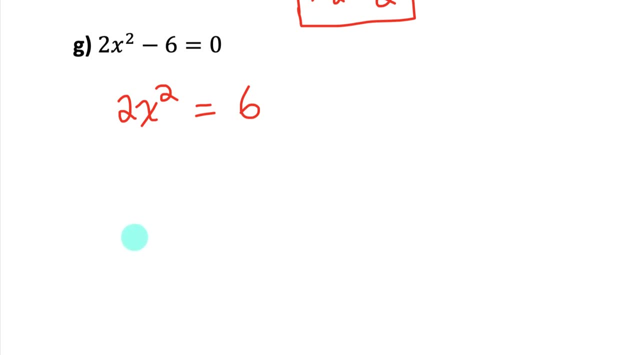 moving the negative six to the other side, It becomes positive six. Then I'll divide the two over Six. divided by two is three And then I can isolate an x that's being squared by doing the inverse of squaring. The inverse of squaring is plus or minus square rooting. 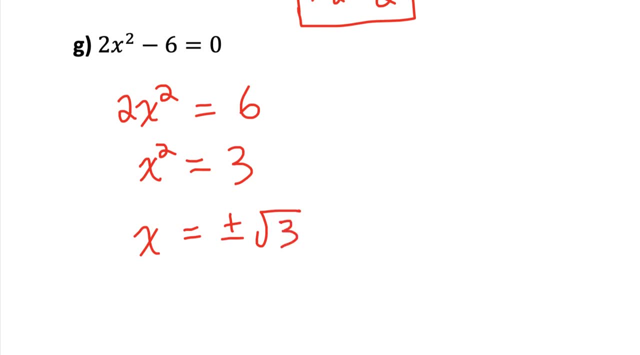 So I actually get two answers for this. My answers for x are positive root three and negative root three. Now you could, I suppose, write them as separate answers, Root three and negative root three. But I would be fine if you just left your answer written as plus or minus root three. 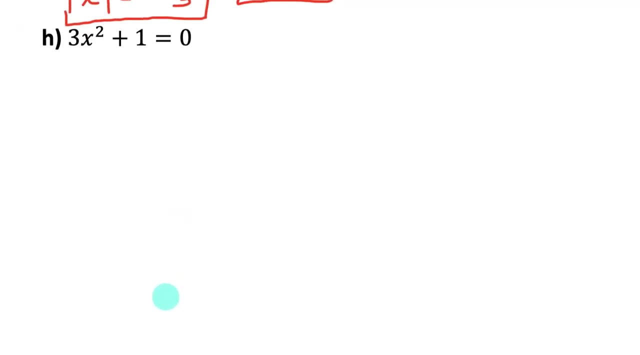 If we look at part once again, it's two terms: The degree two term and the constant. When it's that format, only one of the terms has an x. Just use algebra to try and isolate the x. I'll start by subtracting the one to the other side. 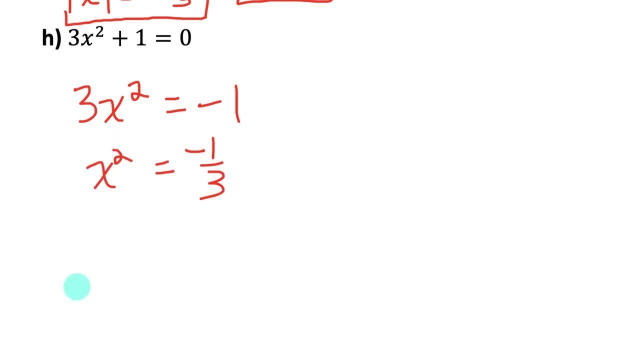 Then dividing the three And then moving the squared to the other side by doing the inverse of squaring, which is plus or minus square rooting. But if we try and square root a negative, we run into a problem. In order to understand why there's no solution, 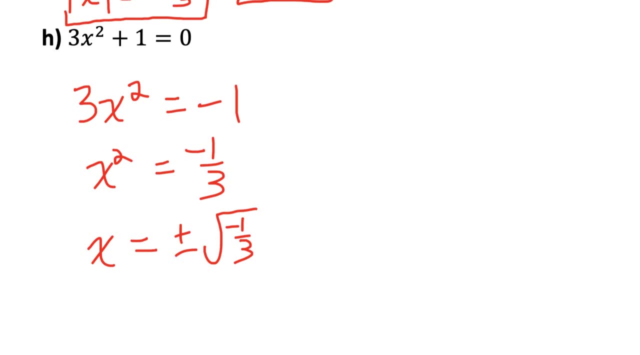 let's just think about numbers that you know how to work with. Like, let's say we're square rooting nine. For square rooting nine, you'd say the answer is three. Why is the answer three? Because three squared is nine. Now think about it. Anytime you square something, it's positive. 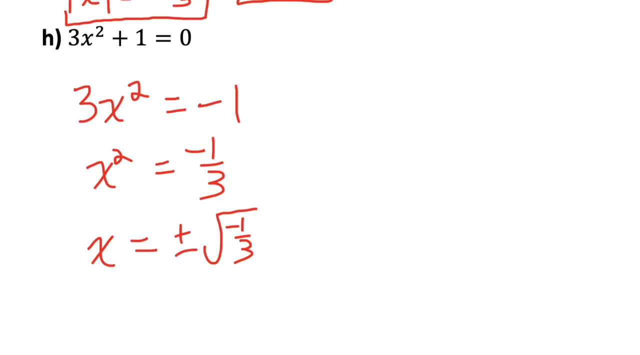 If we're trying to figure out the square root of negative a third, really, what we're trying to do is figure out what can we square to get negative a third. Well, there's no way to square a number to get a negative result. 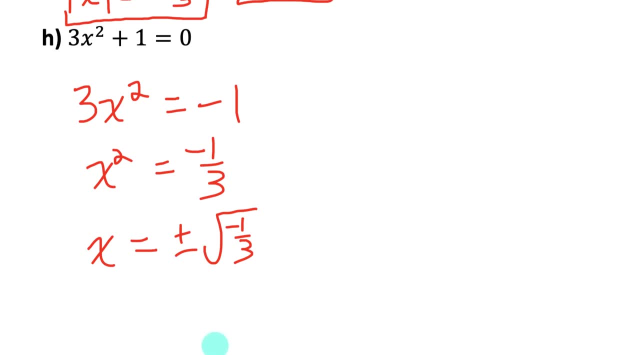 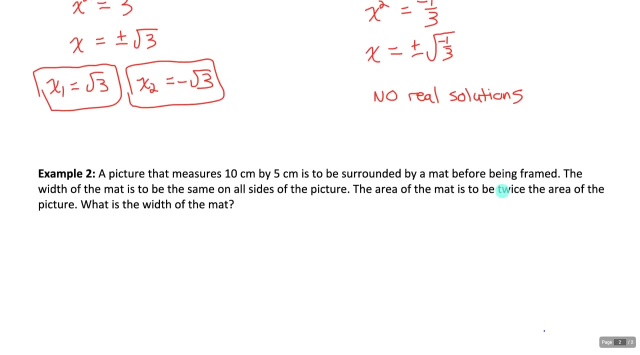 so we know that that's not possible. So when this happens, when underneath your square root is negative, we say no real solutions. Let's now do a quick application question. We have a picture that measures ten centimeters by five centimeters. 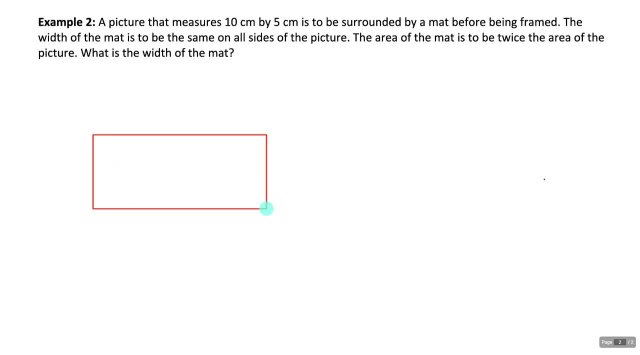 Let me start by drawing that. And it says that that picture is to be surrounded by a mat before it's being framed. So let me just draw a mat that surrounds that picture And it says the width of the mat is to be the same on all sides of the picture. 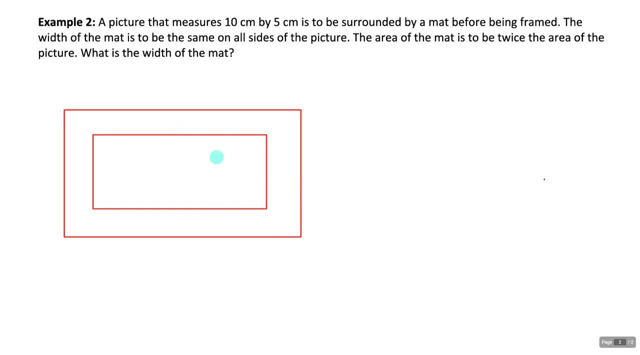 Okay, I think roughly, I made the width be the same on all sides. It says the area of the mat is to be twice the area of the picture. What's the width of the mat? So let's label what we know about this diagram. 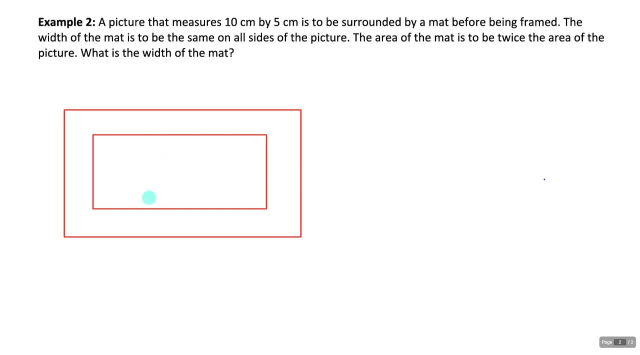 The inside rectangle is the picture And it says the picture is ten centimeters by five centimeters So I can label those side lengths. It then says there's a mat placed around the outside of the picture. Maybe just let me shade in that mat. 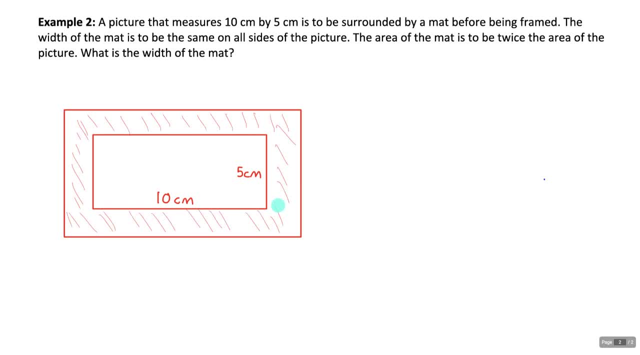 The question tells us that the width of the mat is the same on all sides of the picture. We don't know what the width of the mat is, so I'll call that x, But I know the width of the mat is x there. 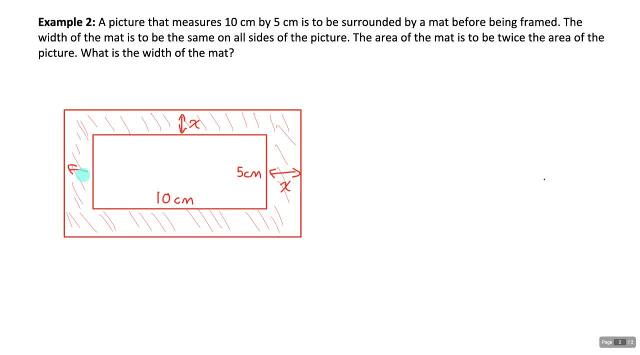 x here. they're all the same, so I'll call them all: x x x. It says the area of the mat is to be equal to twice the area of the picture. What is the width of the mat? So I know the area of the mat is double the area of the picture. 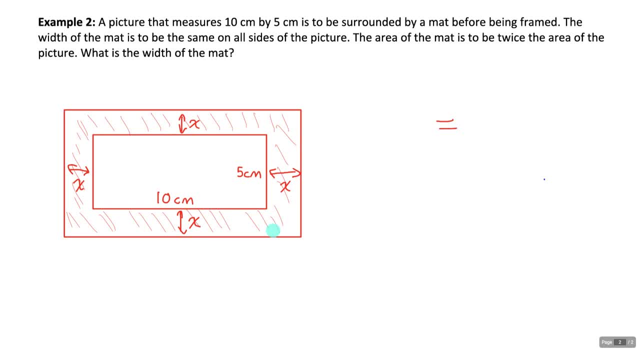 So I'm going to set up an equation: If the area of the mat is double the area of the picture, I know that if I multiply the area of the picture by two- two times picture area- that would be equal to the mat area. 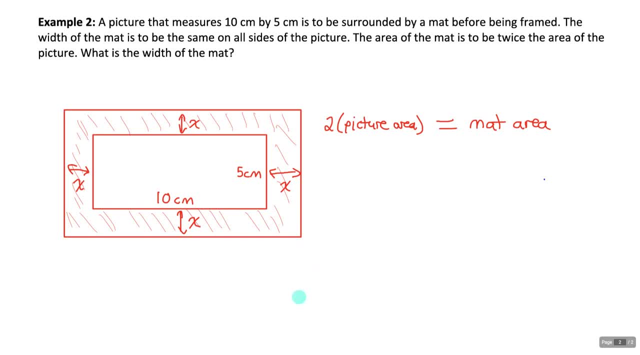 Because the mat is double the area of the picture. if I multiply the area of the picture by two, it should make the areas equal. Now I just need to come up with an expression for the area of the picture and the area of the mat. 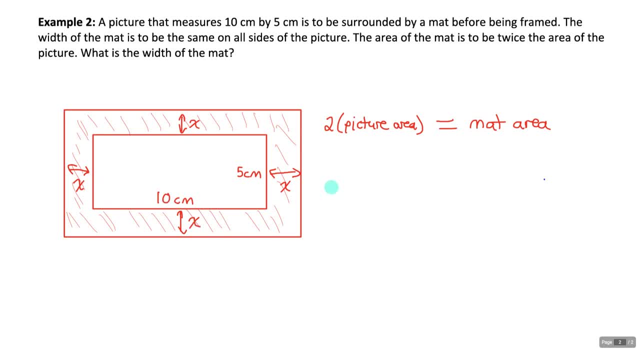 Well, the area of the picture, that's easy. That's the inside rectangle. It's ten by five, So I can replace the picture area with ten times five. The area of the mat's a little more difficult. Let me try and label some different areas. 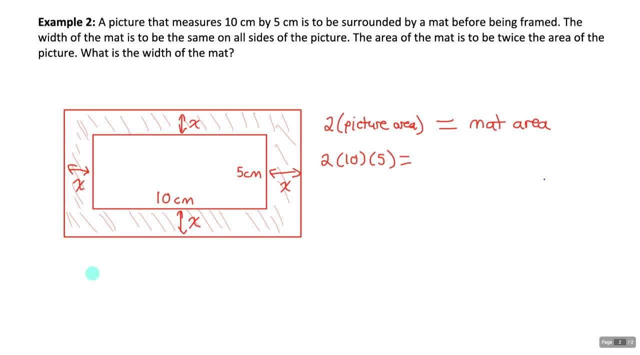 of the picture. So let's look at the dimensions of the big outside rectangle. If I look at the entire length along the bottom, it's ten plus an x extending out from either side of it. So the entire length of the bottom would be ten plus two x. 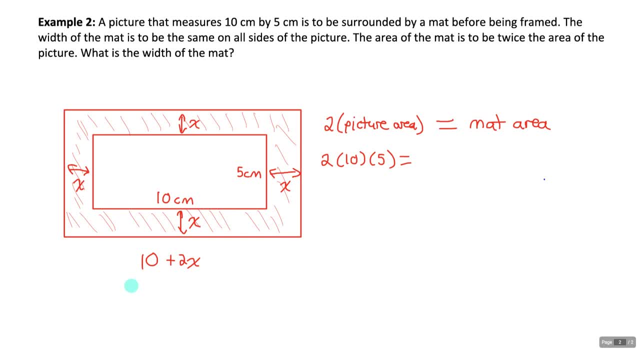 It would be x plus ten plus x to get from the left side to the right side of this diagram. And how would I get from the bottom to the top of the diagram? Plus five plus x, That's five plus two x. So I know the whole big rectangle. 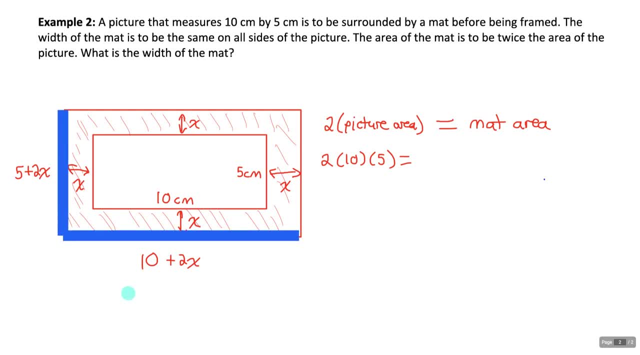 is five plus two x by ten plus two x. That would give me the area of this entire thing. But the mat doesn't exist over top of the picture, It just surrounds the picture. So if I want just the area of the shaded region, 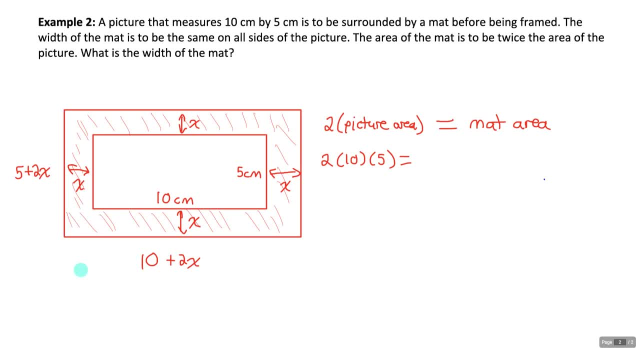 I would have to do the area of this whole thing, the five plus two x times ten plus two x, and then subtract the area of the inside, the area of the picture on the inside, which is ten by five, which is fifty. 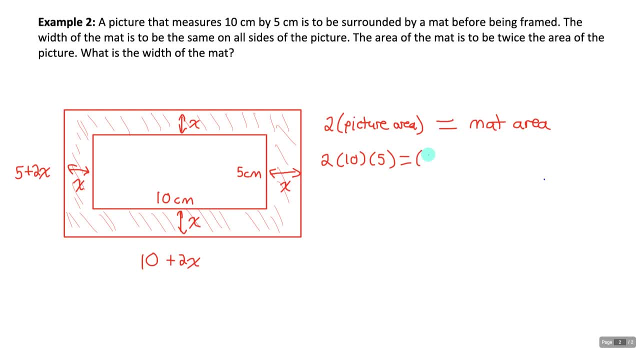 So the area of the mat would be the area of the big rectangle, five plus two x times ten plus two x minus the area of the picture on the inside, which is ten by five. That would give me the area of just the mat that surrounds the picture. 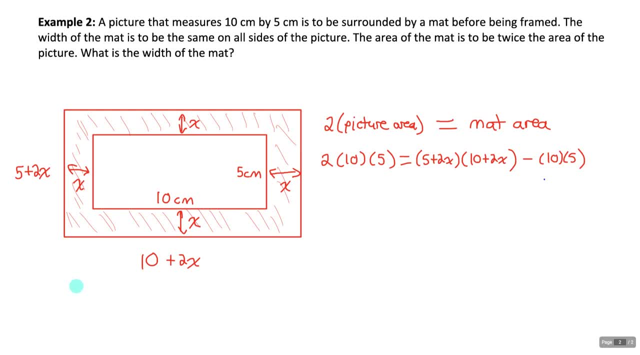 Now I want to solve this equation for x. When we're solving an equation for x, what we're going to want to do is simplify this whole equation by expanding it out, by doing all of the multiplication, move all the terms to one side. 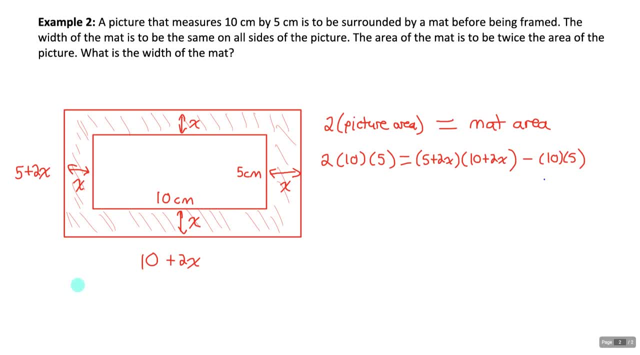 and then see what type of factoring strategy is going to help us solve this. The left side of the equation: two times ten times five, that's a hundred. That's easy. On the right side I have a binomial times a binomial. 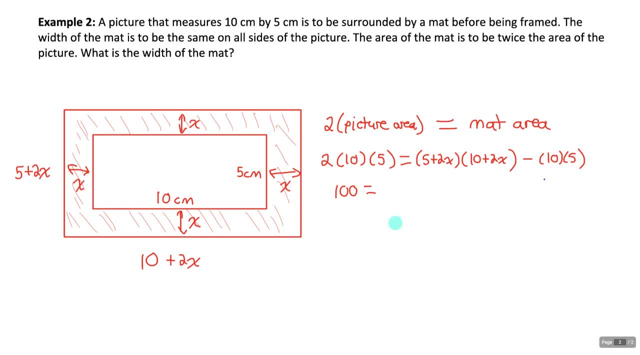 I'll have to use the method of FOIL, which tells me to find four products Five times ten, five times two x, two x times ten, two x times two x. When I find all four of those products, I would have fifty. 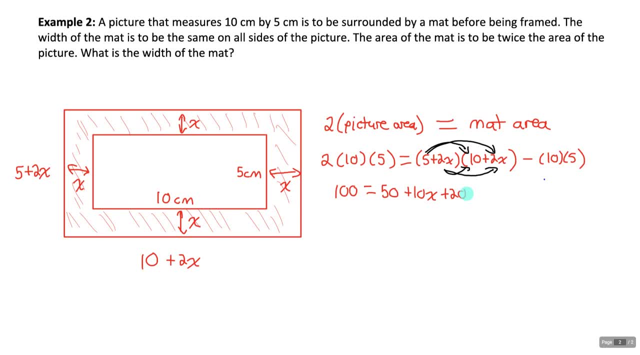 plus ten x, plus twenty x, plus four x squared, minus ten times five, which is fifty. Now I notice this is a quadratic, because the highest degree term is degree two, that four x squared term. Let me actually simplify the right side of this equation. 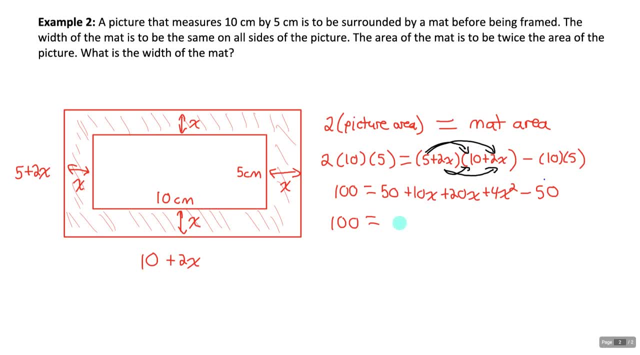 before I do anything. On the right side I have a fifty minus fifty. those cancel out, that's zero. I'm going to rewrite the four x squared and I have a ten x plus twenty x, that's thirty x. Now I'm going to want to set this quadratic to zero. 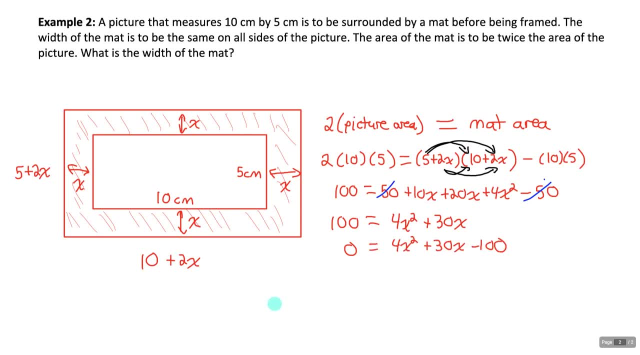 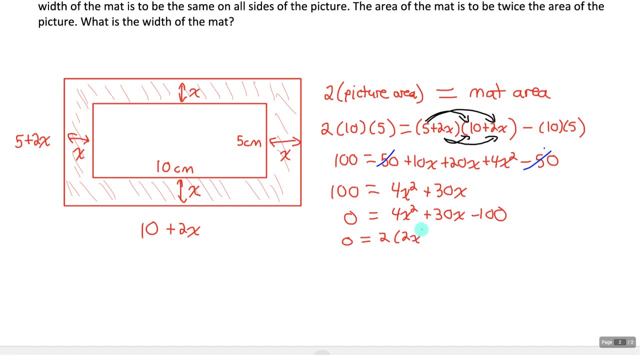 So I'll move the hundred to the other side. it becomes a minus a hundred. And then I'm going to want to solve this quadratic. First of all, I notice all three terms are even, so I could common factor out a two from all three terms.